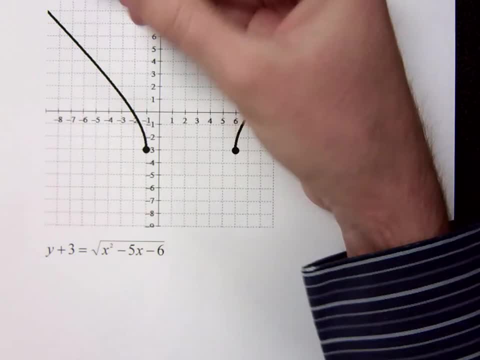 Oh, more than a point, Which is two points or more. No matter where I draw it, It has to go down at least once. but what about that section where there's nothing? Am I going through more than a point? More than one point? 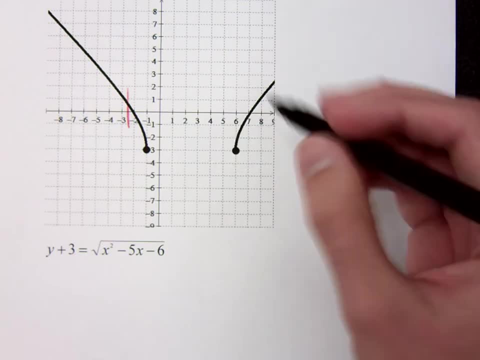 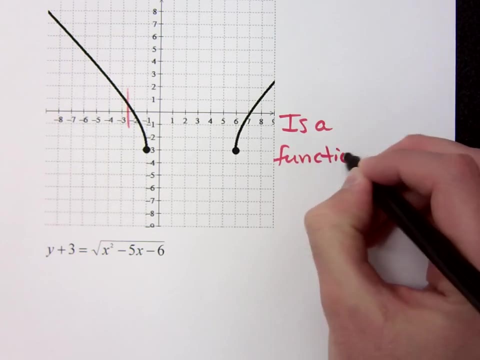 No, no, Then you're okay, So it's good. It's good, So it's a function. This guy is a function. This guy is a function. I can't draw. that Is 6 passing through 2? It looks like it. 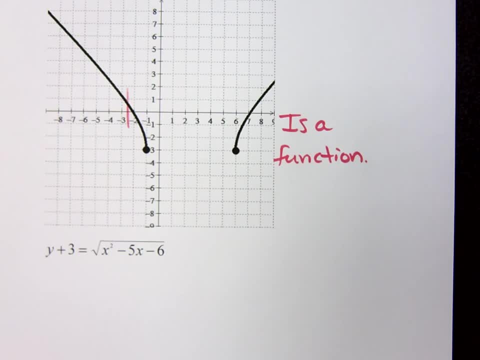 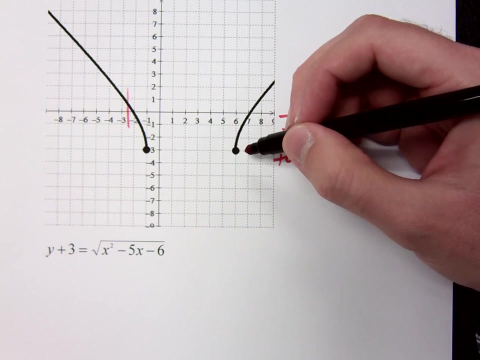 I mean negative 2? Is 6 passing through Negative 3.. Negative 3. Because it looks like it's hitting negative 2 and negative 3.. You have to understand that what we have here is a picture. It's a picture that's generated from a computer. 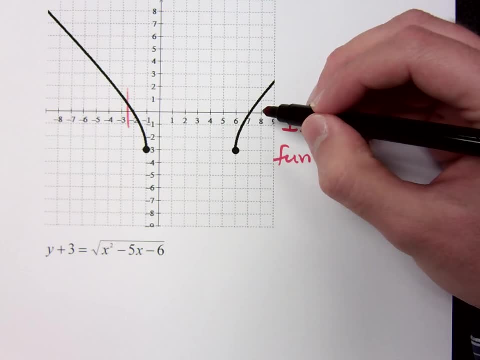 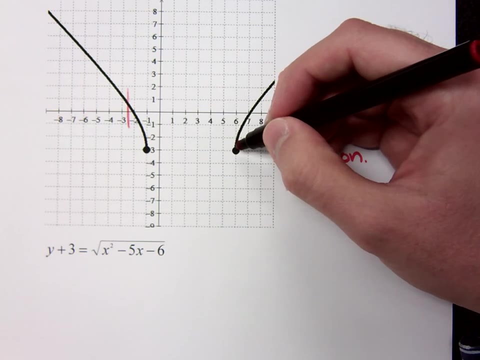 And so it's doing its best to draw it as accurately as possible. So there may be the illusion that pixel-wise, vertically, there would be more than one point. But this guy starts here and he is getting further and further out here. 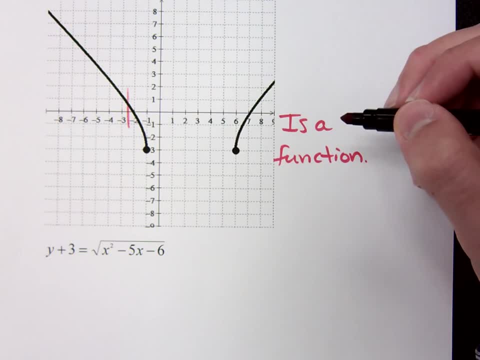 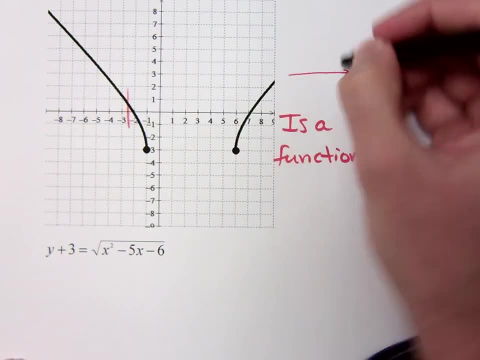 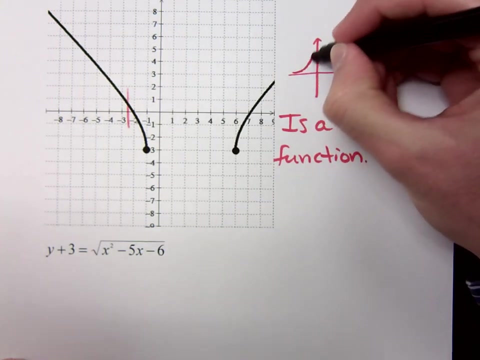 You just have to understand that certain things that we can't see very well will be true, Like we may see things later on that do this. I will have in college algebra something that does this. This guy gets closer and closer and closer to this. 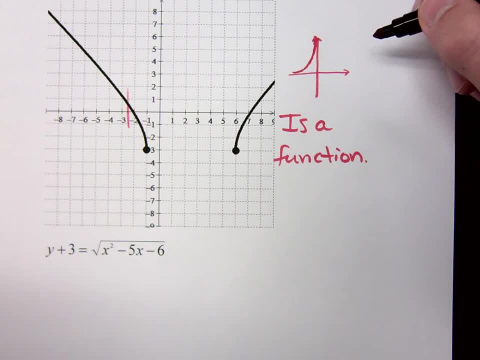 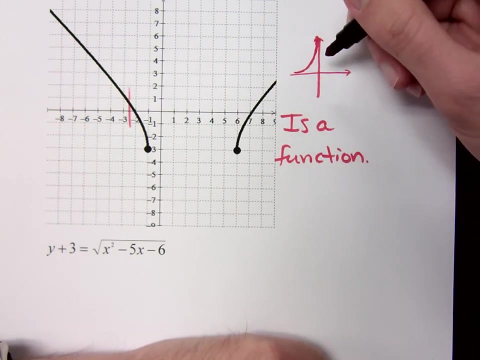 It looks like it goes vertical, but it never is straight up and down, Never. So the changes are very hard for us to see, because you can get really really close to this and you can make it look vertical, and over a short distance it may be that way. 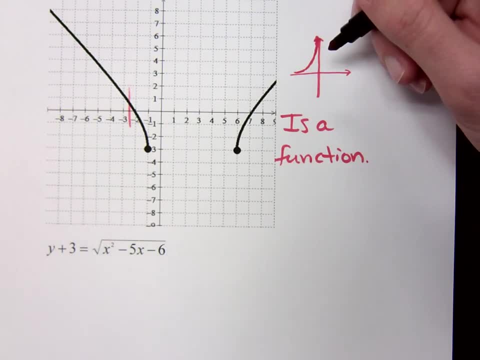 but it is never, ever vertical. I just want to make sure so we didn't, you know, get like a trick question or something. It would be indefinite. No, no, no, You'll know for certain that it's not going to be a function. 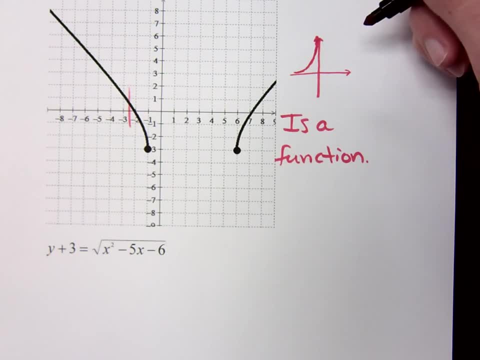 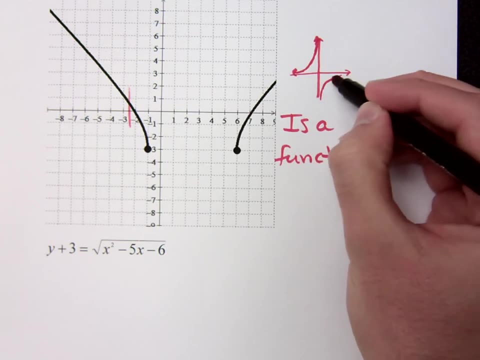 Like the last example, there was an oval Or an ellipse, excuse me. Yeah, Now this guy is a function. Even if I did something like this, this guy would be a function. You may see something like this later on. 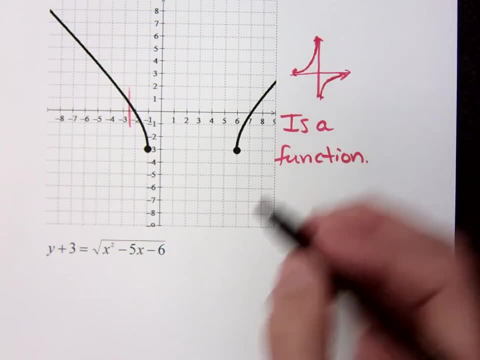 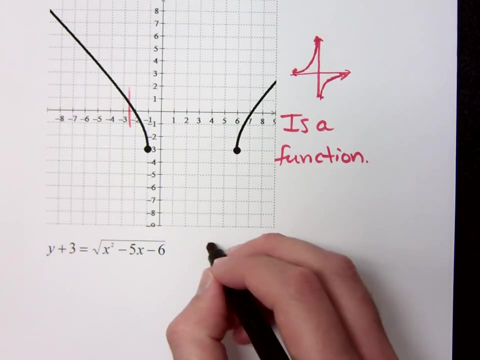 Because is it a function? It passes the vertical line test. If you draw a vertical line that goes through more than one point, it's not a function. Now let me ask you this: What is the domain? And I guess I should put this here for you guys. 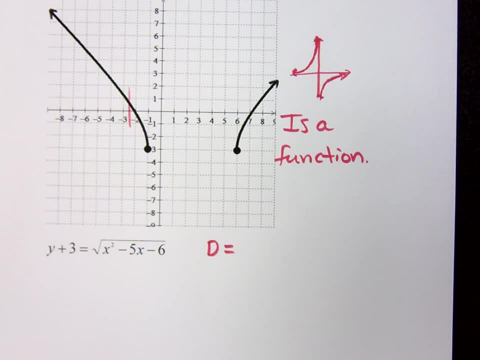 This does extend forever in both directions Like that. Okay, I can't get the arrows to show up very well. whenever I print this, Do you put a bracket on it and then negative. You never put brackets on infinity or negative infinity, So parentheses. negative infinity. to what? 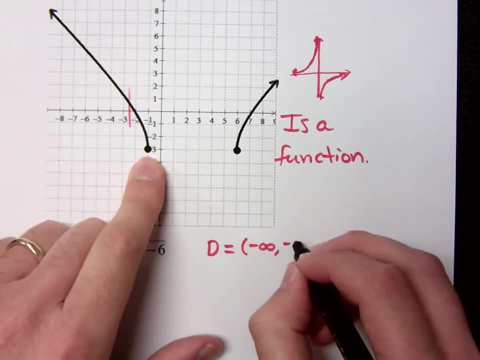 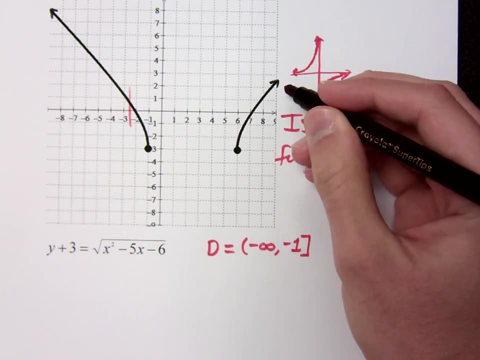 Negative one and then bracket Negative one and then get a bracket here. But that's only for this part, right? Right, But I have this other part, that's also part of my graph. So what do I do? Bracket six to infinity. 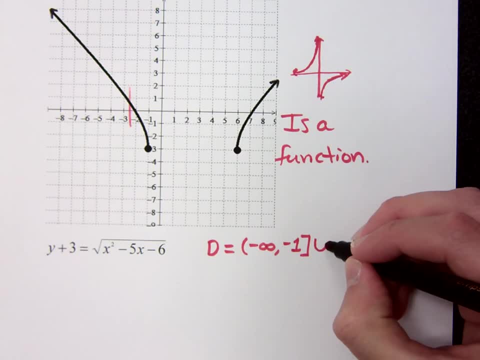 Right Before I can get there, though, Cliff Use that union symbol because I'm joining those two guys, So then I do my bracket six to infinity, Just like that Six. Now, here's what you need to understand about this guy right here. 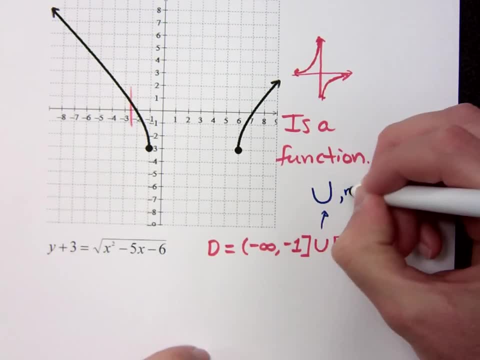 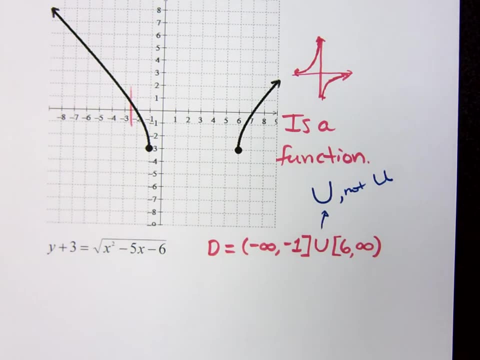 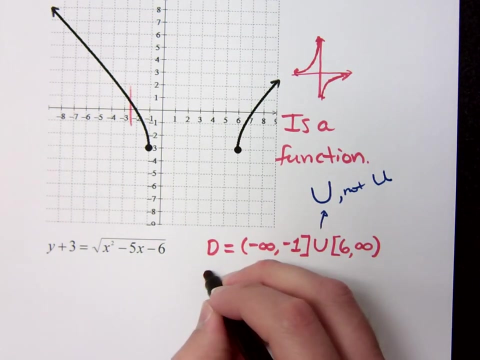 This guy is the union symbol, not this guy. Don't make it like the letter U with a tail or you will be wrong. It's just the symbol for the union. Now, what about your range? Range is from least to greatest, bottom to top. 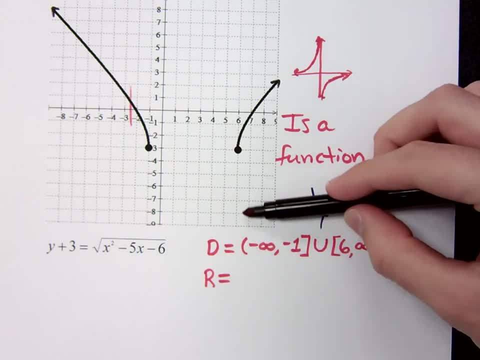 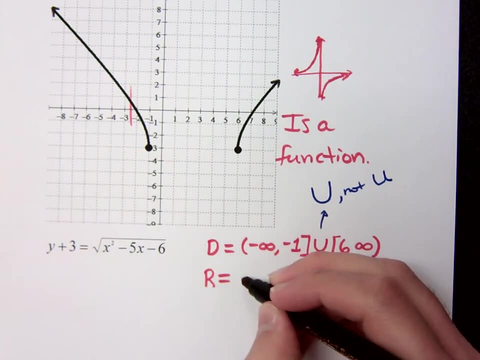 What's the furthest down? this guy is Negative three Right. He starts at negative three, Including negative three Right, Because you see I've got the closed circles there. Negative three to what? Infinity, Infinity. You're looking at this from a vertical perspective. 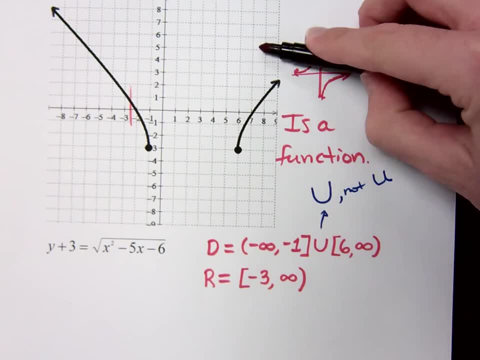 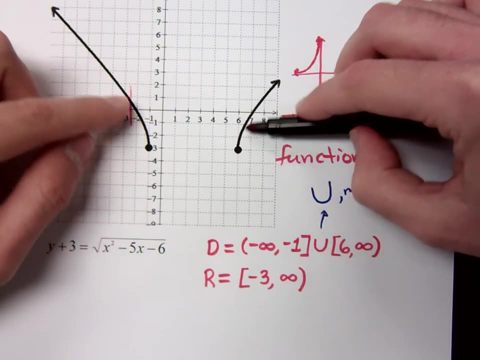 You're starting from negative three and this guy goes all the way up, Even on this side. Don't think about him going up to the left. We're talking about from a vertical perspective. So we start at negative three and these guys are both going up all the way.